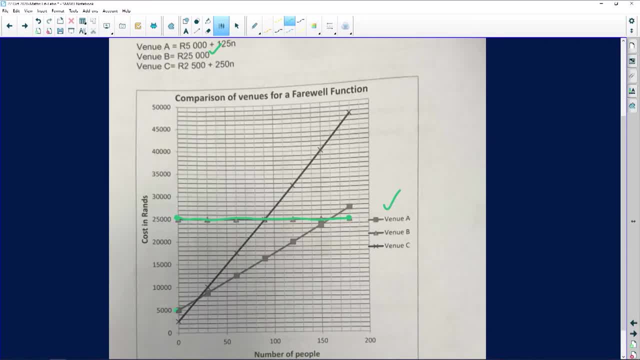 I'm going to show you the other one. The last one is venue C. Venue C is the one that almost looks spiky, Starts here and it ends over here. Now, these two graphs guys, This graph and this graph- I would call them direct proportion graphs. 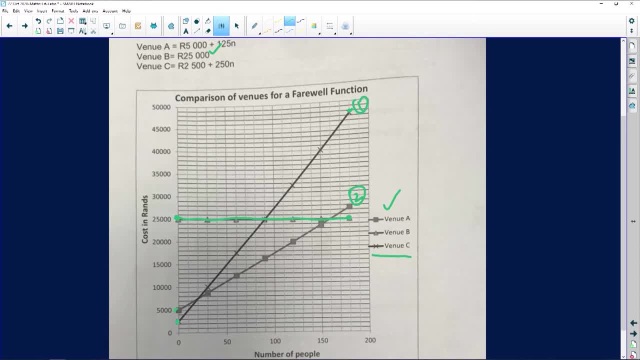 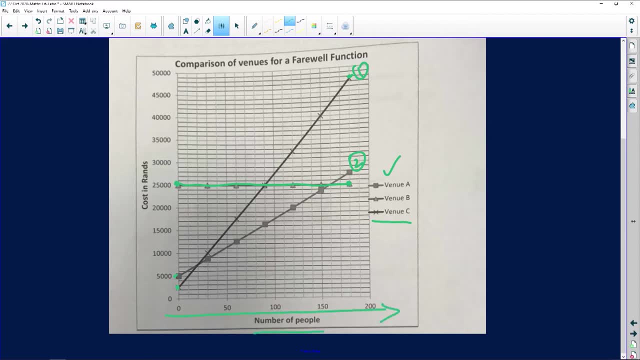 Why are they direct proportion graphs? Because as the number of people increase, as the number of people increase going that way, the cost also increases, going up there. So it's constant. But you can see, let me not go too much into these graphs- 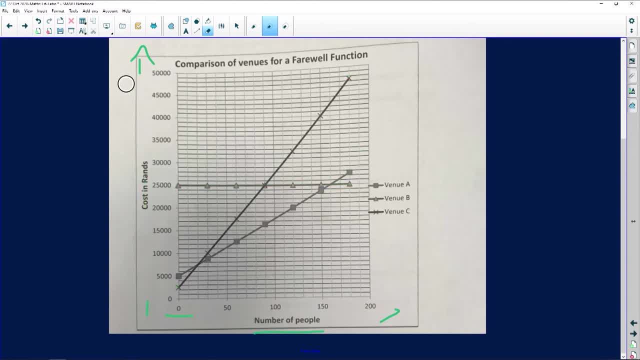 Let's go answer before We run out of time, because I'm getting ahead of myself. I just want to make that clean for us. Okay, So that was just me. now I've got my graph there. I'm going to read now all the questions that I need to read concerning this particular graph. 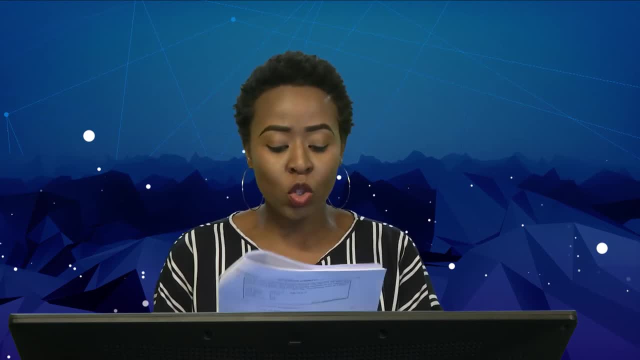 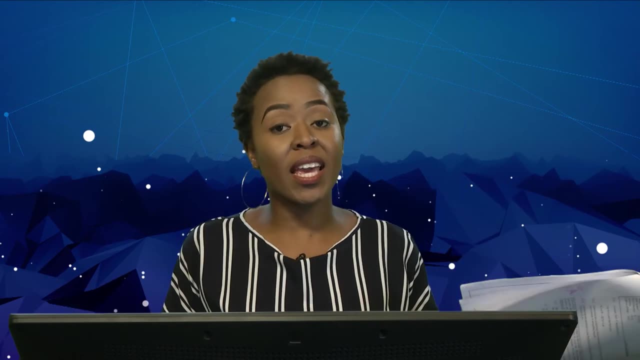 The first question says to us: how much will it cost for hosting a function At venue A for a hundred people? In this particular case, all you're going to do is trace on the graph. We're going to go to a hundred people and trace it up to the mani. 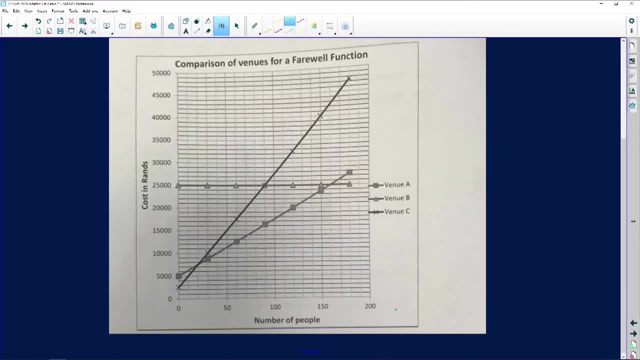 Okay, So this is a hundred people and we're looking for venue A, So we're going to go up until we touch this graph and then it's going to tell us the amount of mani. So a hundred people. I'm going up, up, up. 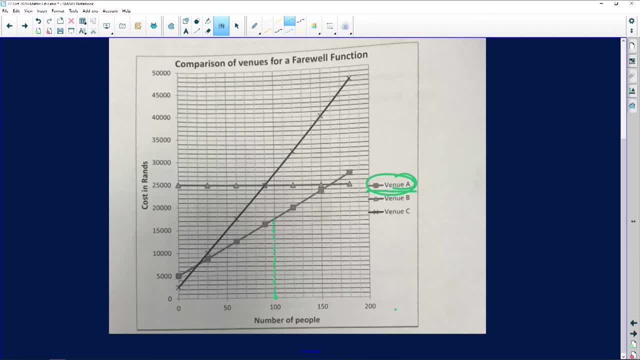 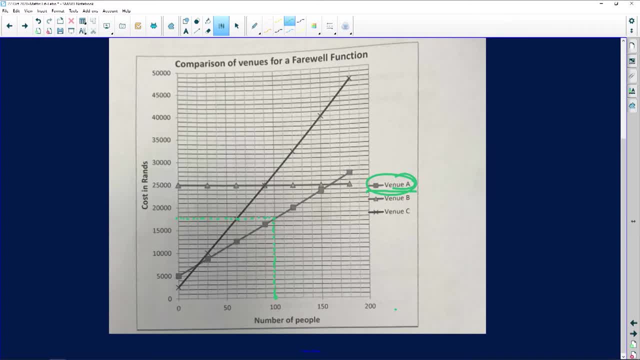 to do now. so it's going to be halfway- i hope i am correct- two, two years, halfway between um fifteen thousand and twenty thousand, so i would say halfway between fifteen thousand and twenty thousand. this graph is going up in. let me see two, four, six, eight, ten. it's going up in twos, so in: 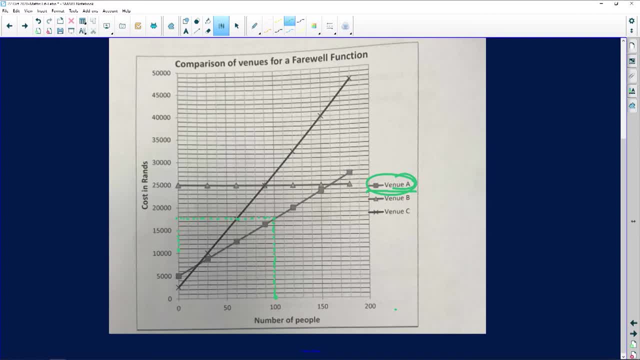 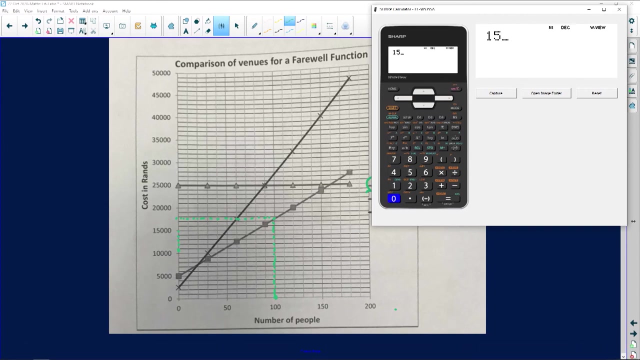 this particular case, um, it's fifteen thousand, so i would say that it's going to be um fifteen thousand seven hundred and fifty. that could work, but it might not work. let me see something like that with the calculator, a little bit of trial and error. fifteen thousand plus twenty thousand. 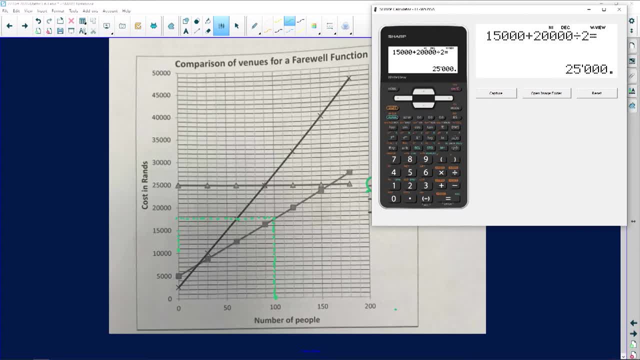 divided by two. oh, actually, no, i did something wrong. something is not correct here. it's fifteen thousand one, two, three, divided by twenty thousand one, two, three equals two divided by two, three, seven, five. okay, that's not really working out for me, but i choose that i am going to use. 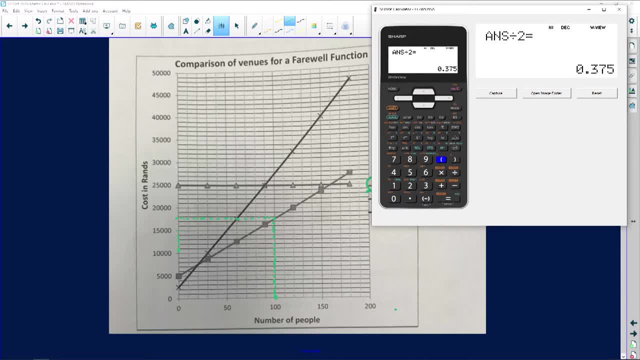 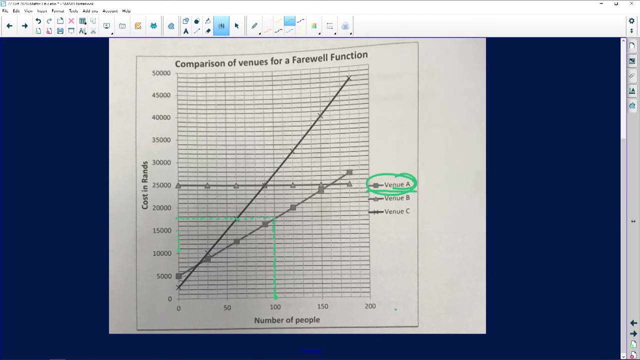 what is halfway between fifteen thousand and twenty thousand. it's going to be eighteen thousand, okay. so it's going to be um, eighteen thousand, okay, thank you so much for that. so it's going to be in between, so i'm not going to make it eighteen thousand. it's going to be seven thousand, seventeen thousand five hundred. okay, because it's. 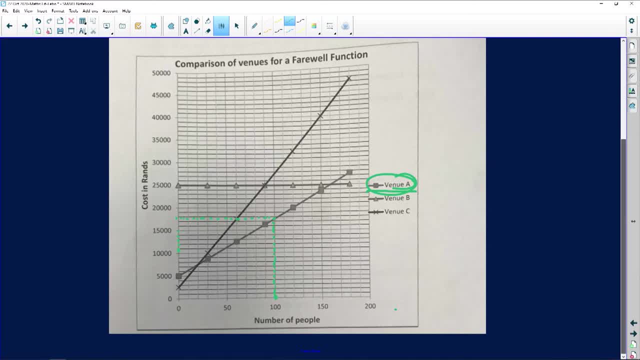 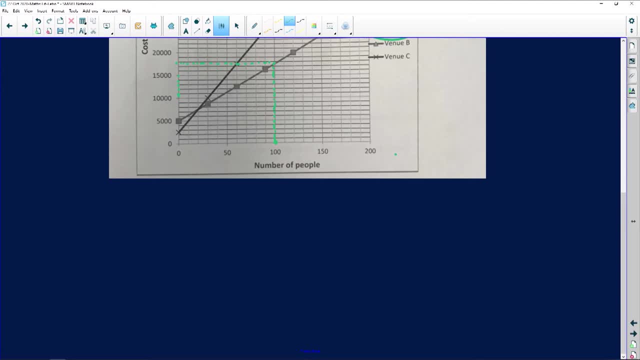 all the way in between. thank you so much. i got a little bit of help over there, so in terms of that it's going to be seventeen thousand five hundred rand. um, that i am working with seventeen thousand five hundred. i got dribbled for a moment over there. thank you so much. 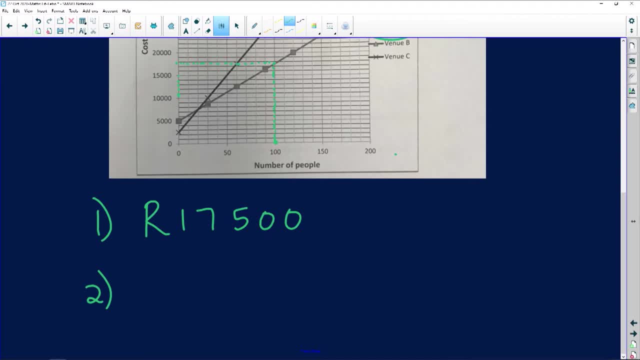 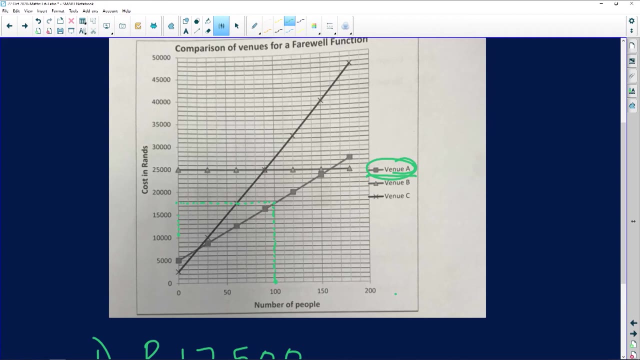 so the next question, um that we are working with says to us: identify the most expensive venue to entertain one hundred and eighty people. so what we want to do is find where one hundred and eighty is going to be. so this is one hundred and sixty, seventy, eighty, ninety two hundred. 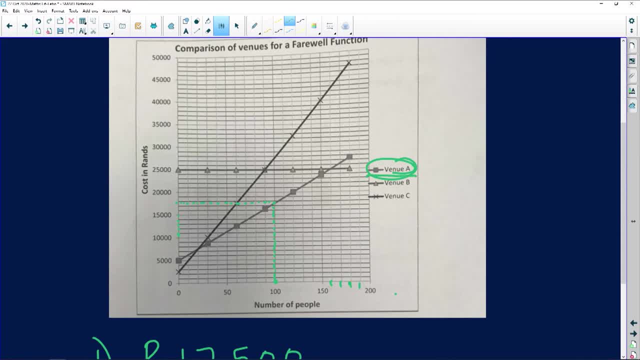 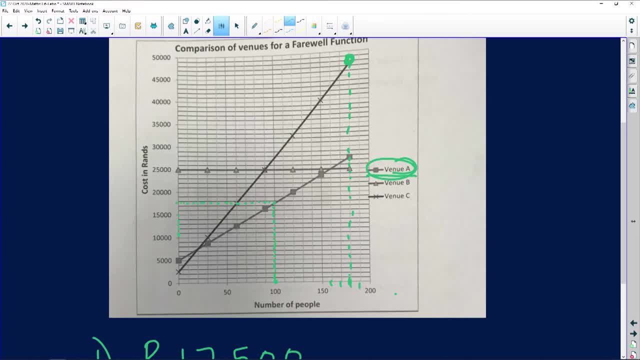 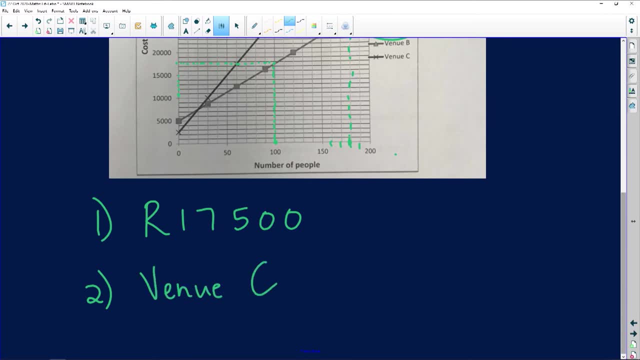 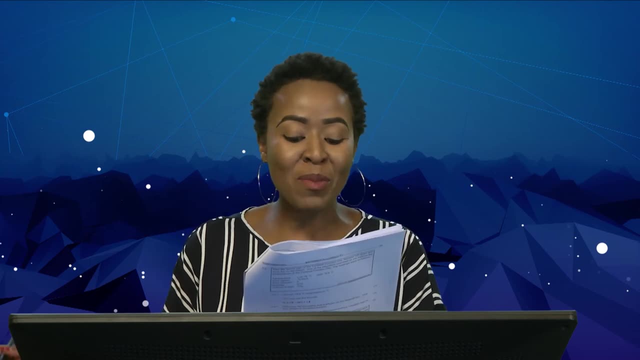 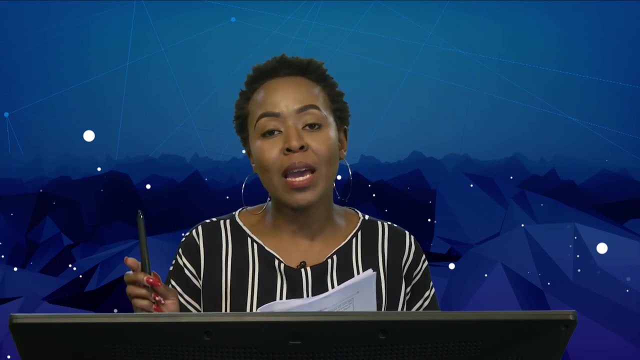 is going to be the most expensive venue because it's above the other venues. so it's going to be venue c, number three. number three says to us determine the number of people that can be hosted for four thousand rand at venue c. so every time they talk about people, i'm going up. now they're talking. 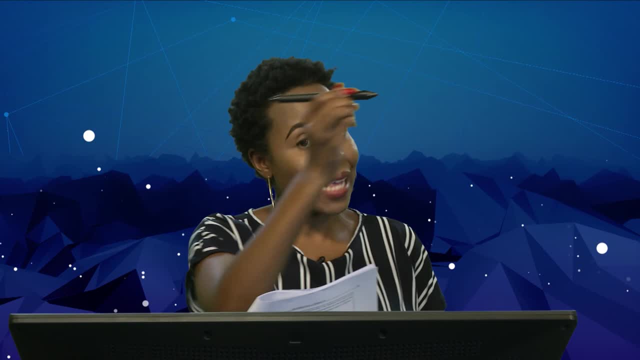 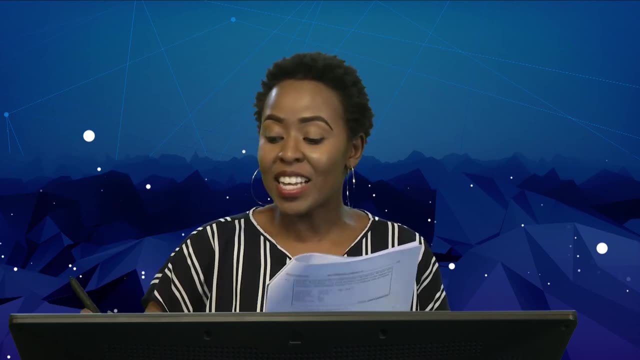 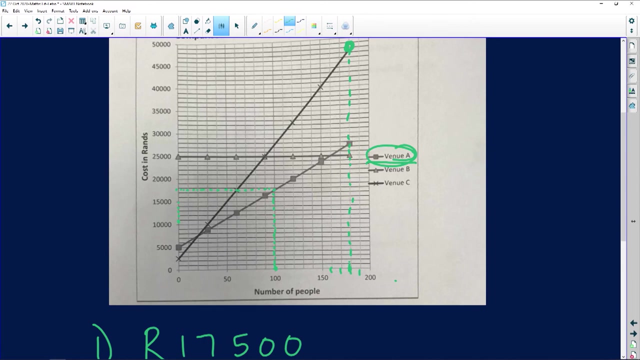 about money. now i'm going to go from the money sideways until i touch um c and then it's going to tell me how many people are going to be needed. let's go to five. point one. point three: so it says to us: here for four thousand rand, four thousand rand, guys. so this is going to be one two. 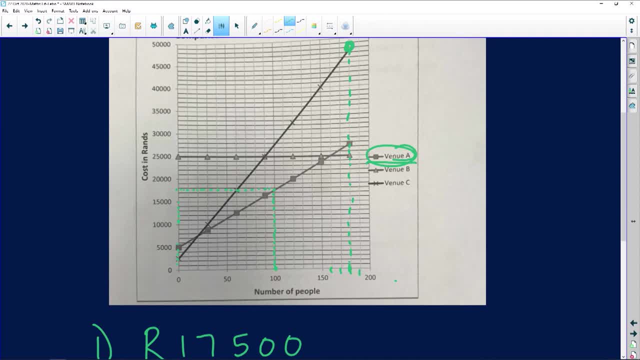 three, four, five, so four thousand rand is going to be over here, and then i'm gonna go until i touch c. c is the spiky one, so this is c, and then c is going to be us going down halfway again. oh, this graph. okay, So this is 50, so I'm assuming it's 10,, 20,, 30,, 40,, 50.. 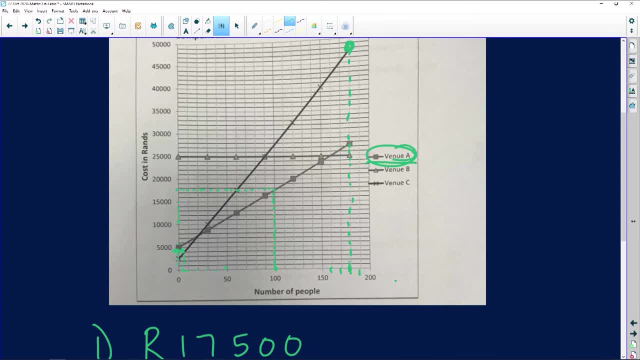 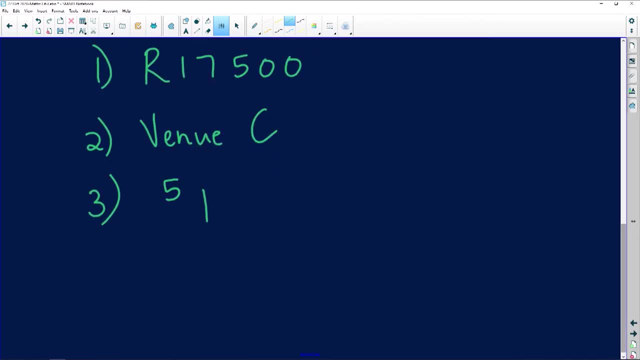 So it means this venue will be able to accommodate five people, because this is in between zero and 10.. Five people And honestly also, it means for every five people you're going to pay 4,000 rand Number four. number four says to us: 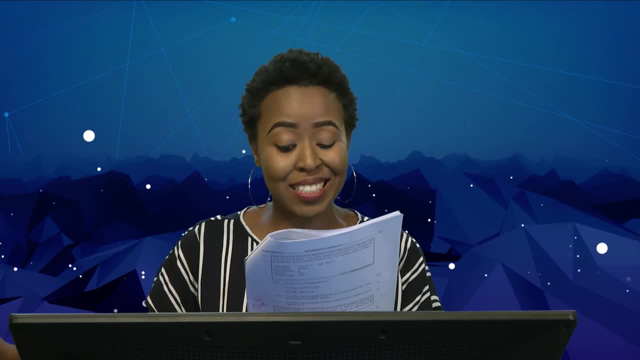 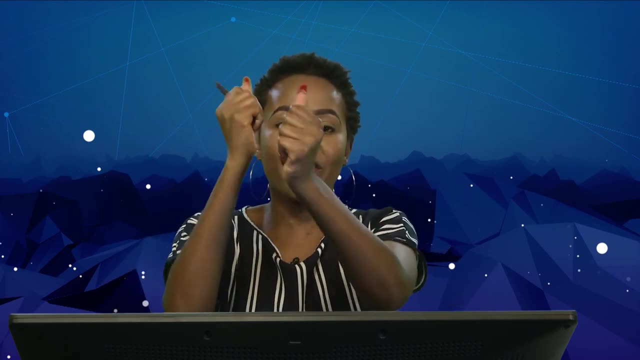 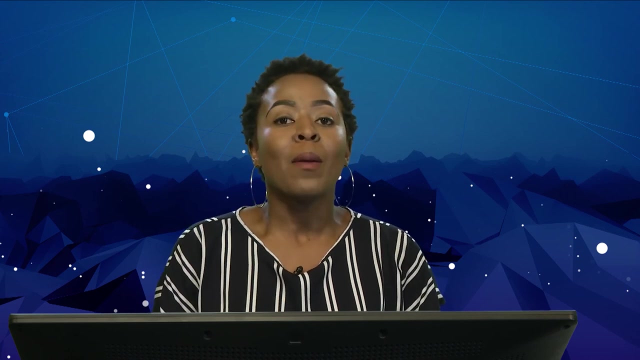 write down. write down the three intersection points of the graph. So intersection is where the graphs meet. okay, Wherever the graphs are meeting, that's the intersection. So this graph, apparently, according to what they're telling us, meets at 3..